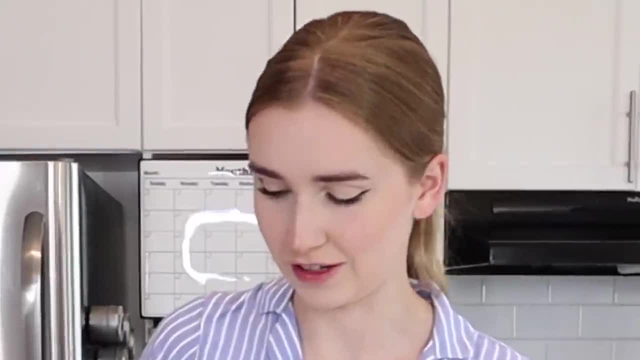 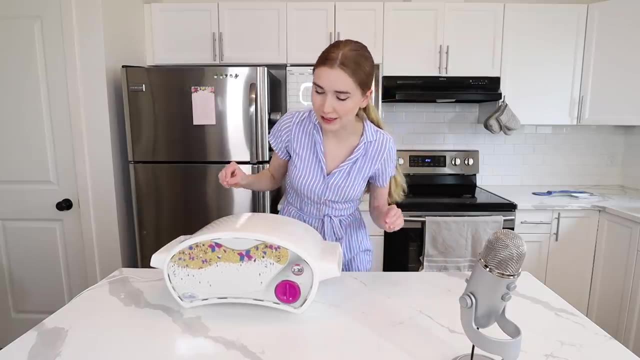 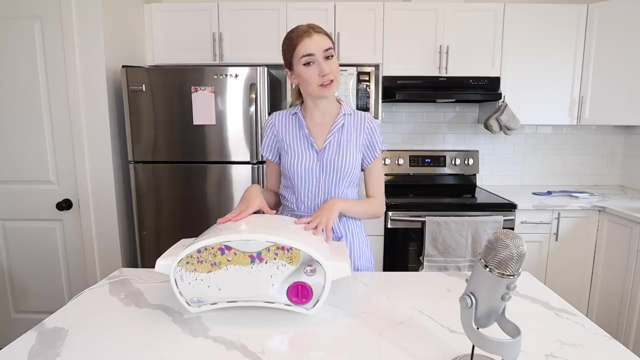 I loved my Easy Bake Oven so much. Oh my goodness, I made such a mess of my Easy Bake Oven. When you would look in the slot you would just see like dried burnt cake, but it was amazing. I was reading an article that said Easy Bake Ovens got discontinued this year. Is this true? So basically, 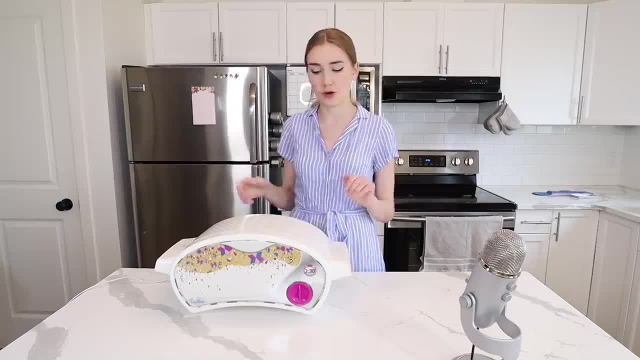 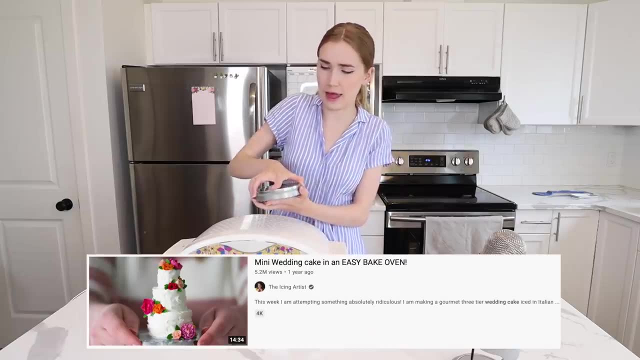 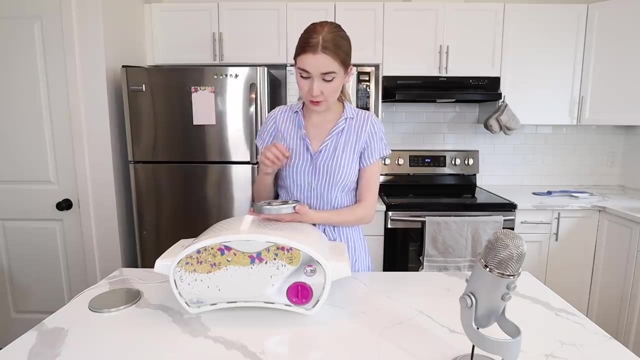 I was watching cake videos, as I do, and I've seen so many people play with the Easy Bake Oven. One video in particular caught my attention, and it was the icing artist made a mini wedding cake with her Easy Bake Oven and I was like: so that's what we're doing today. 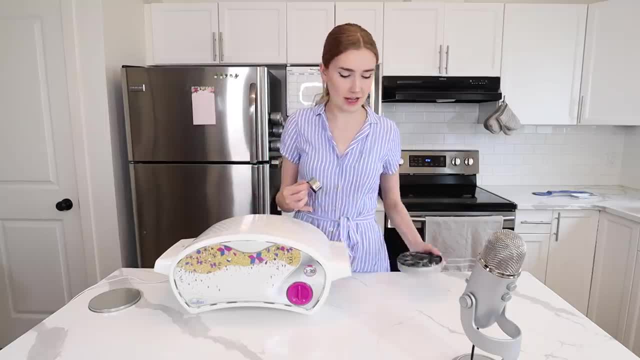 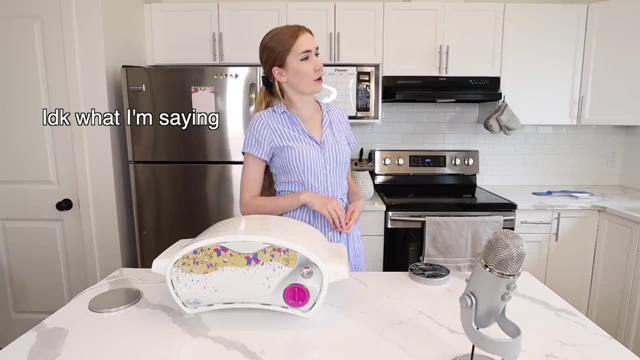 Isn't that cool- Except not a wedding cake. I'm just gonna make a three-tier fun cake. I actually have these cookie cutters which are gonna work perfect. This is going to be the size of our cake. Practice makes perfect. 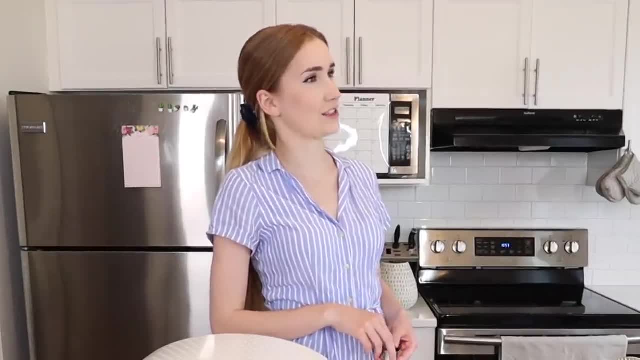 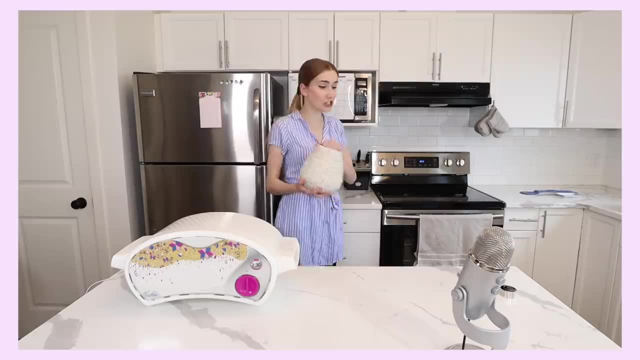 Effort is great And I am excited to eat this cake in one bite. So let's begin. Before we get into this, we have to do the donation portion really quick. Let's pick a charity: The Make-A-Wish Foundation. 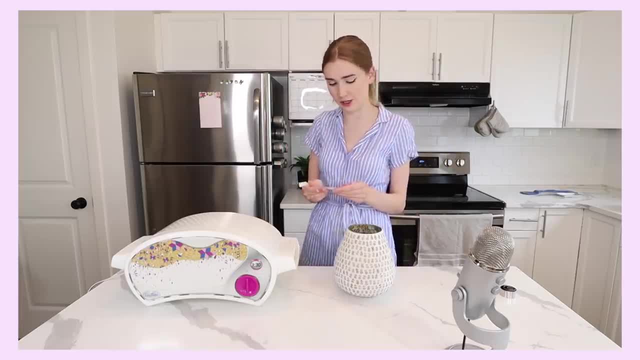 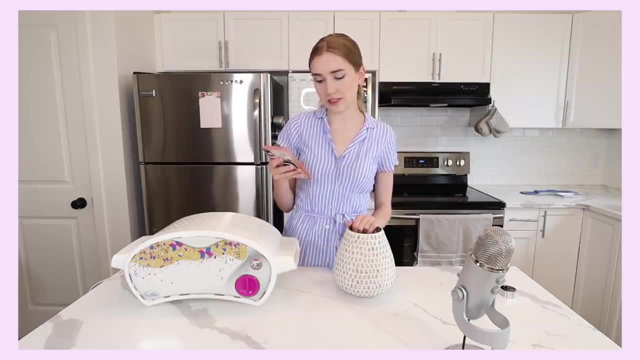 I mean, this charity was commented, so so much, This is a great charity. I'm sure a lot of you guys have probably heard about Make-A-Wish, but here's what they write on their website: Make-A-Wish works with communities across the country. 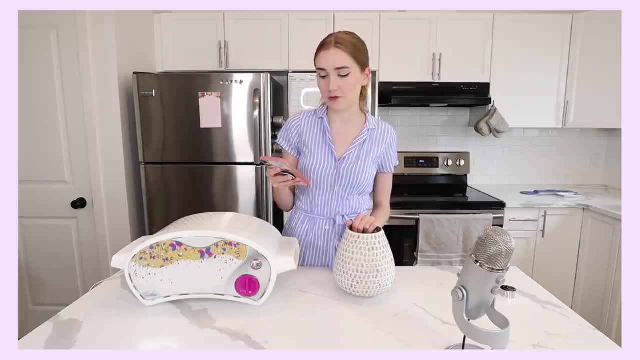 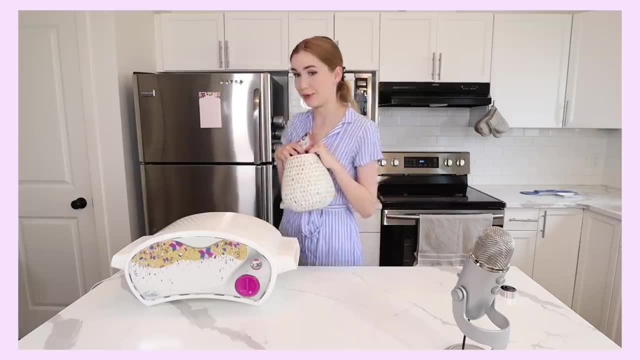 to provide children with critical illnesses the opportunity to realize their most heartfelt wish. So an amazing charity. That's gonna be the charity for today's video. Now let's get into the Easy Bake Oven. Okay, for starters I'm gonna turn this on. 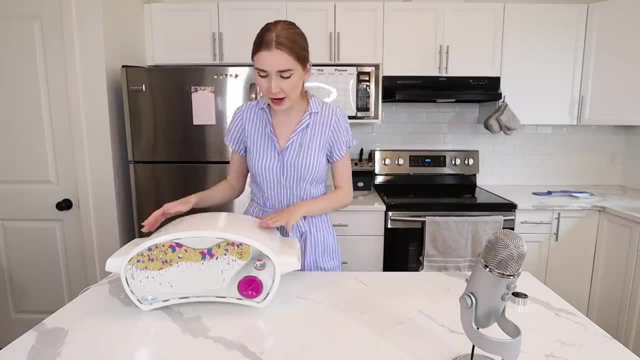 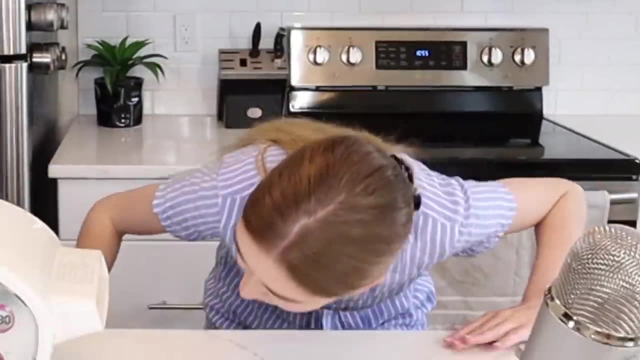 because I think it needs to preheat. It's weird, because the one I used to have had a little window where you could watch the cakes baking. This one they just go into this machine and then I can't check on them. Okay, in our Easy Bake Oven. 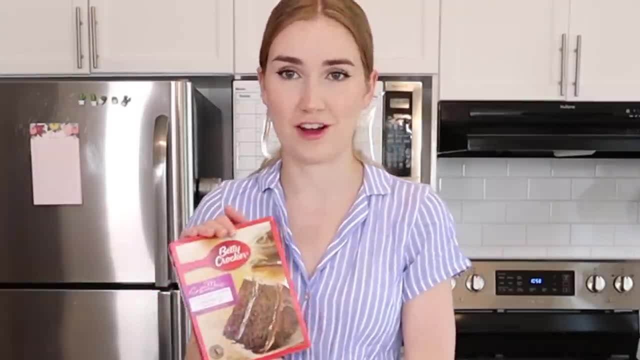 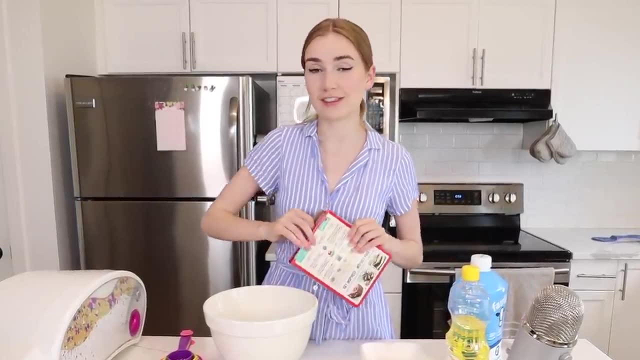 we're gonna be making this Betty Crocker Super Moist Chocolate Fudge Cake Box Now. one day, very soon, I will stop making cake boxes and start making cakes from scratch. I'm always surprised with how much oil are in these cakes. 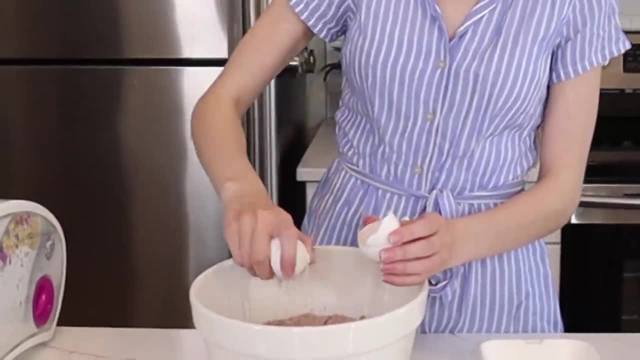 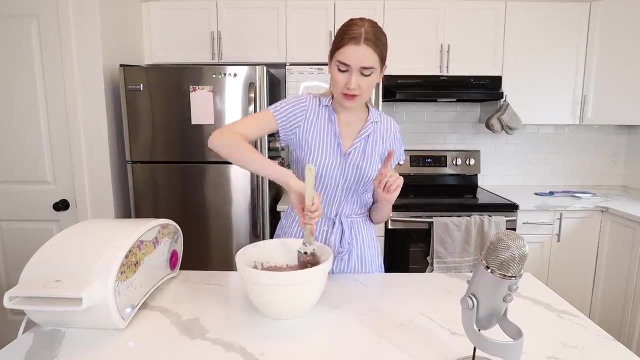 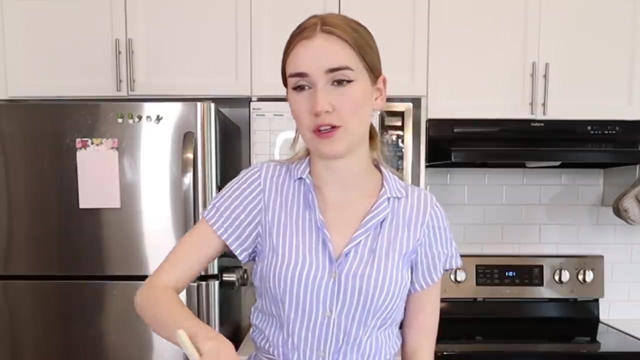 Should I try and one hand it? Oh my gosh, I'm actually so impressed. I don't think I've ever done that before. I honestly have the goal for this video that I eat the entire little mini cake in one bite. It just feels funny to put like four hours of work. 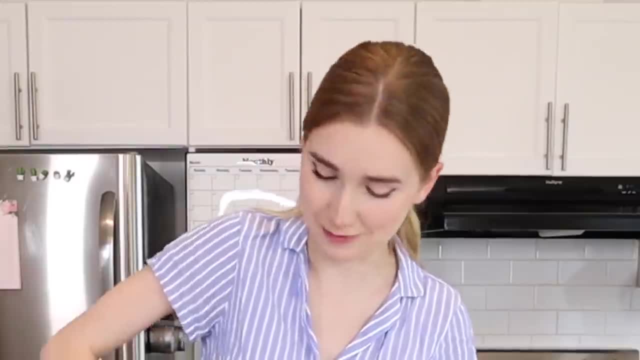 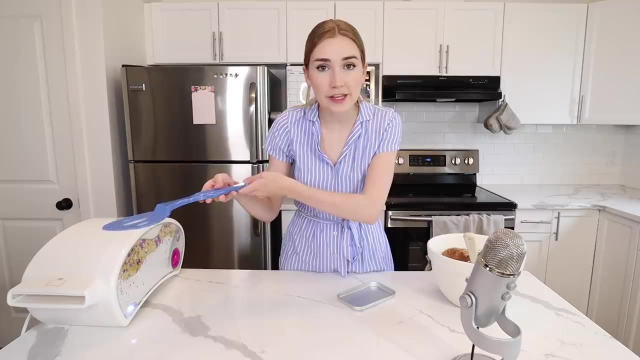 into a little mini cake and then eat it in one bite. So I wanna do that. Okay, to the side. Okay, here are the tools that come with the Easy Bake Oven. We have this, which is like what you push the cake in with. 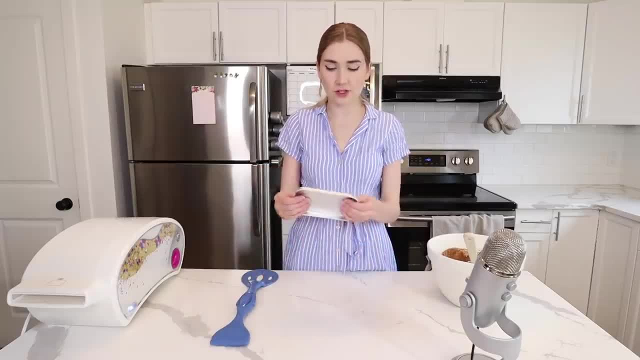 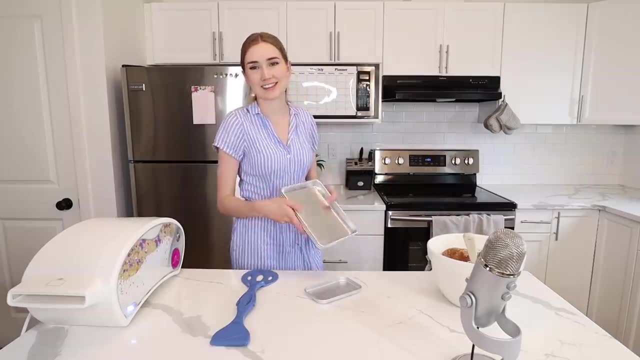 And then I think what you grab the cake with, And also one of the tools that comes with the Easy Bake Oven, is this one tray. Now, I don't know why, but I thought I would buy a few more trays, but I didn't check the size. 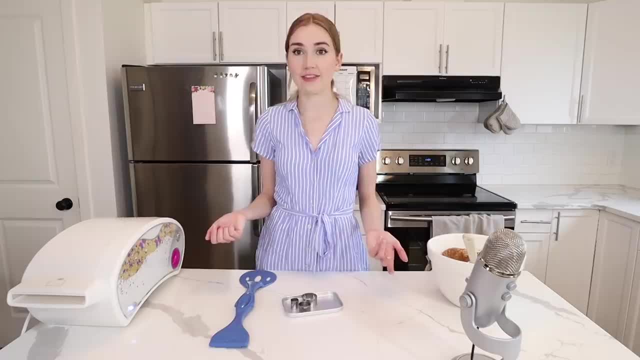 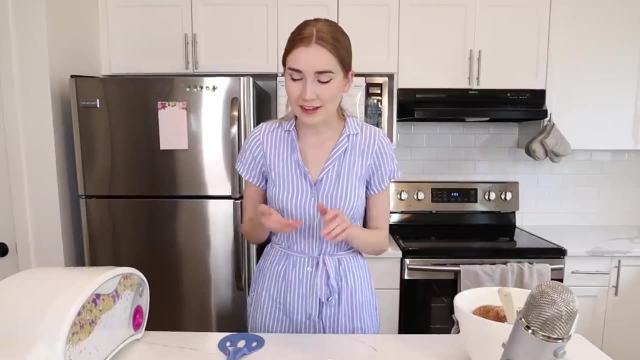 So we'll do for sure two, And then we're actually get this. I never layer my cakes, And you guys always comment about that. Well, today is the first day we're gonna try and layer the cakes, And what an amazing day to try that. 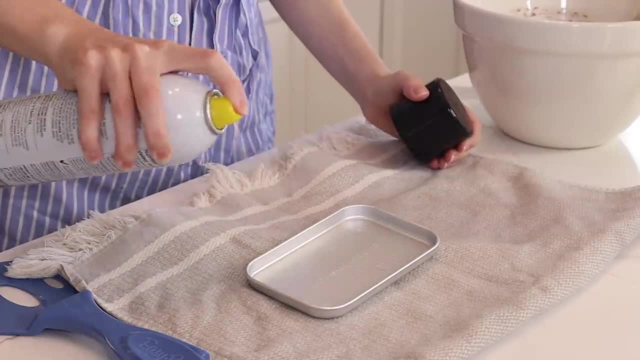 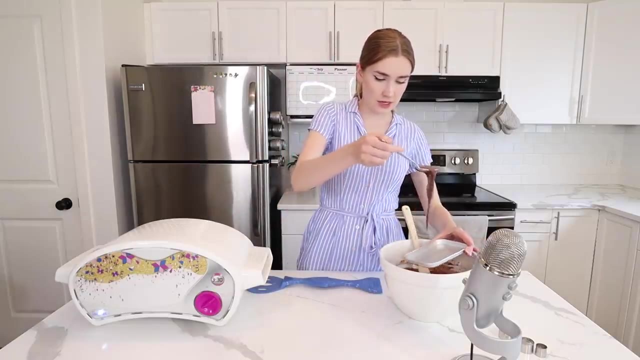 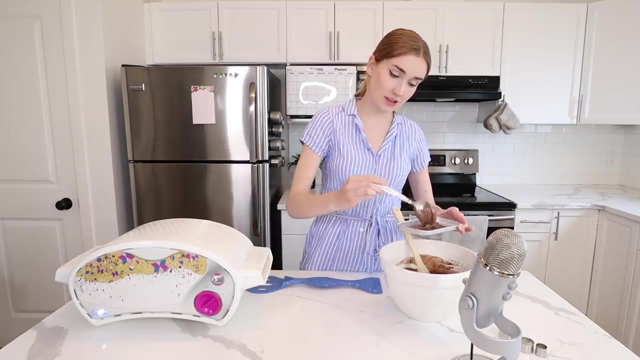 when the cakes are this big, Because the last thing I want is my cake sticking. It's so big. It's time to fill the tray. The Easy Bake Oven is preheated. I don't know how full to fill this- Like not even a clue- but I know that this was a problem when I was a kid, Filling these way too. 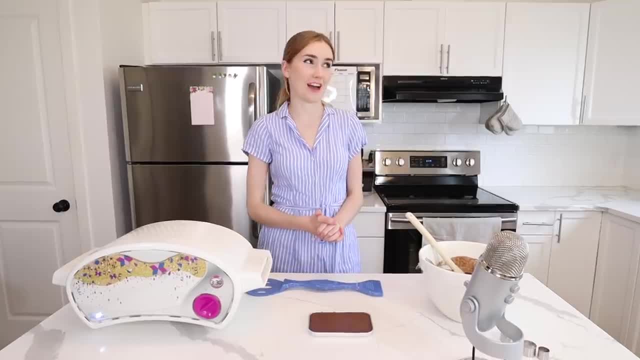 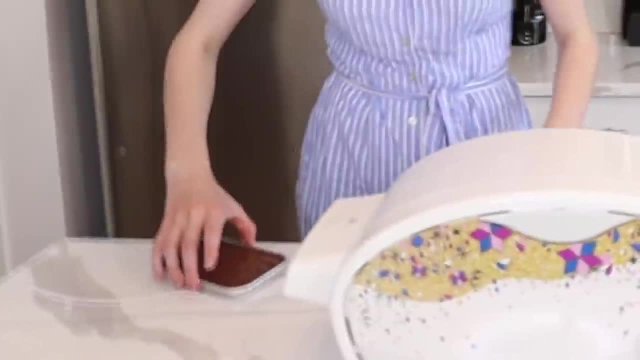 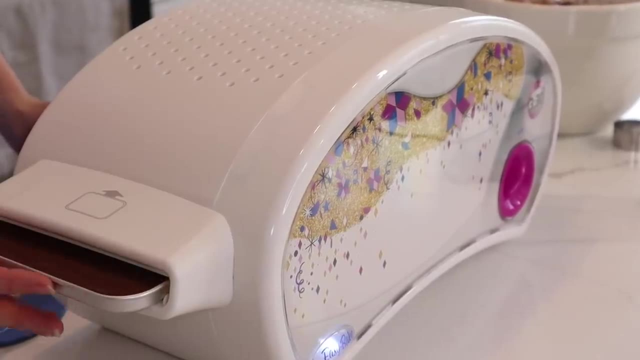 full. Oh my gosh, I'm so excited. I'm having weird flashbacks to when I was like seven years old, doing this on like a Saturday morning. I can remember it so vividly. This is scary. Okay, my Easy Bake Oven has preheated for 20 minutes and now I'm going to push it in. Oh my gosh, Oh. 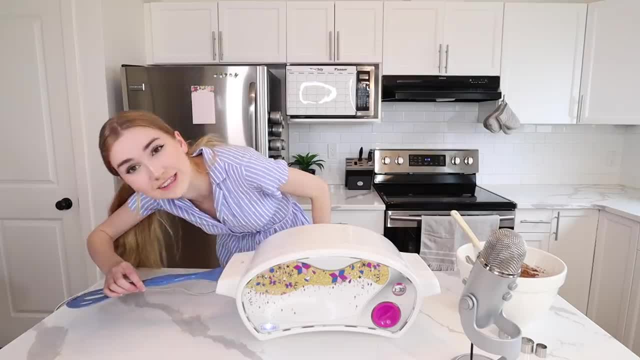 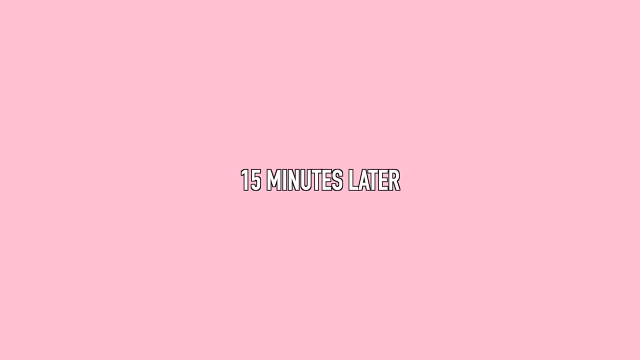 my gosh, How do you know? How do I know when it's in good enough, I think it's good. Oh my gosh, It's cooking. Everyone remain calm. It smells like it's burning. I need to see What does it. 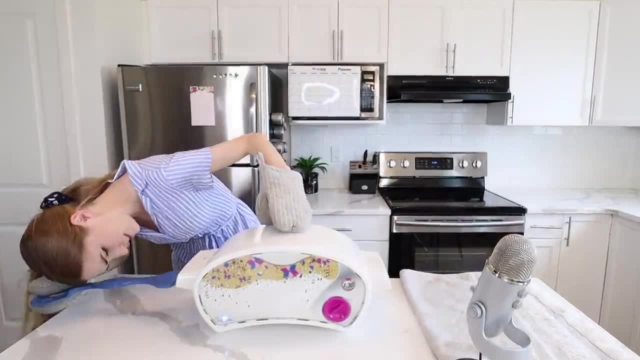 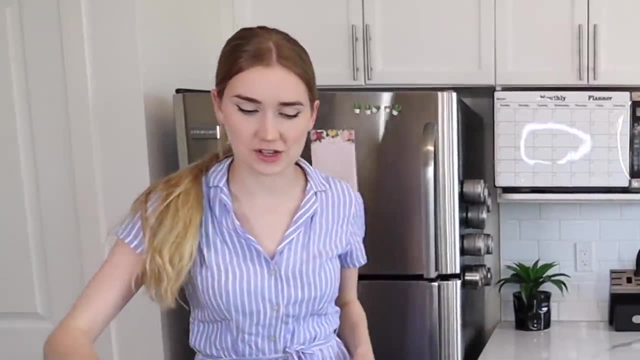 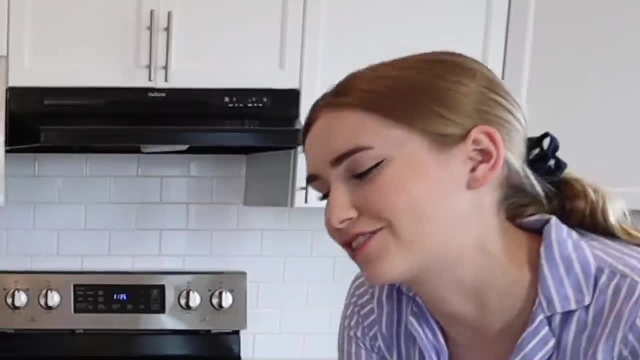 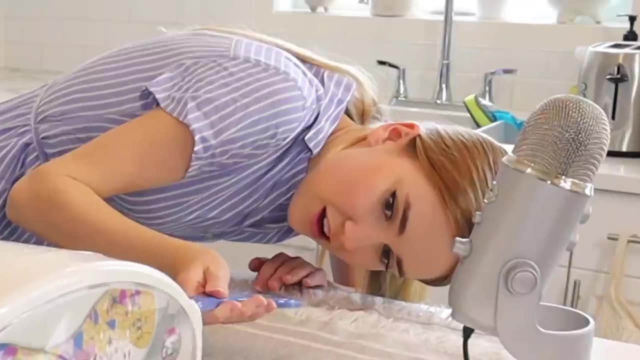 my gosh, Oh my gosh, Oh no, It's too tall, It's way too tall. This is exactly what used to happen. Okay, I have it, but it's so tall. Give me my cake. Oh no, Get out of there. Get out of there. 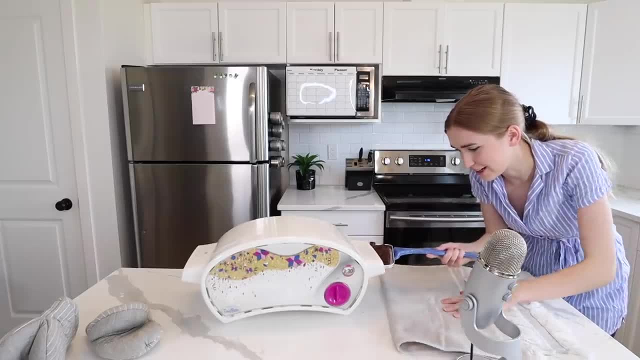 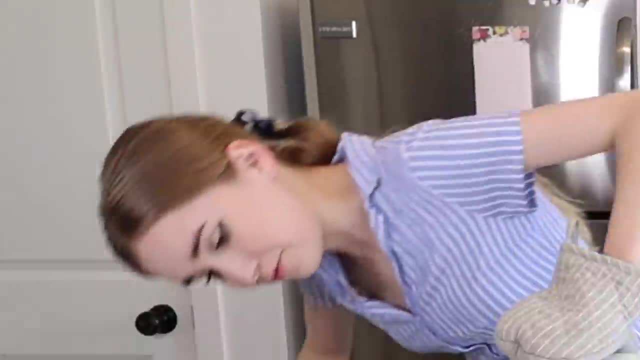 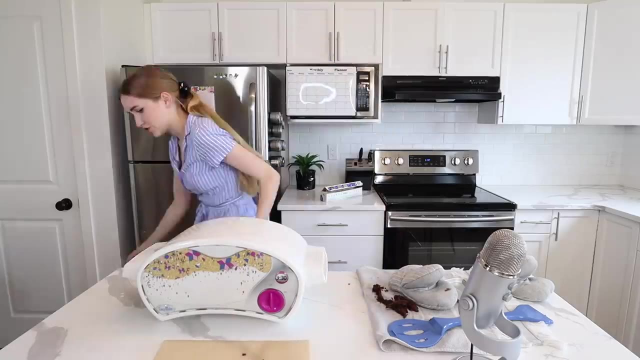 Oh, no, Bad things are happening right now. My easy bake oven is full of cake. Oh, there's cake everywhere. Okay, That actually doesn't look too bad When I show it like that. it's not too bad, but I kind of want to try again, just because I. 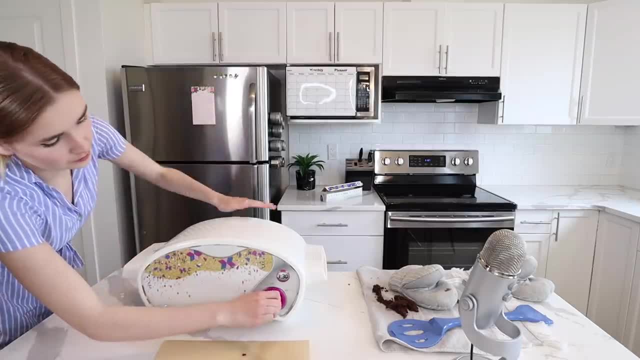 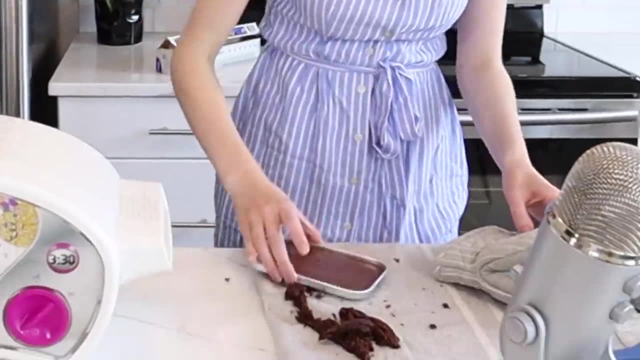 feel like I didn't push it in enough. Okay, I'm going to guess it's already like preheated enough. I just grabbed this fresh out of the oven and it's not even that hot. That could have been really bad. Okay, So like not full at all, I'm going to push it in far enough this time. Oh my. 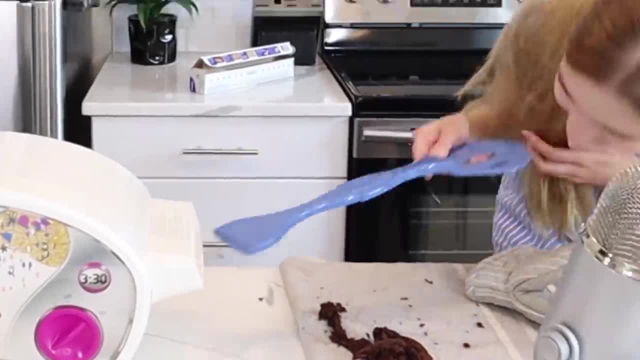 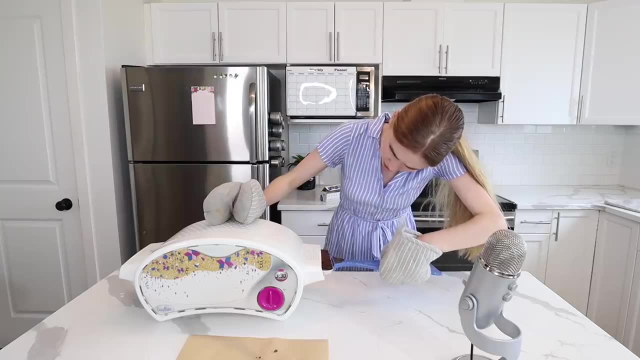 gosh, Oh gosh, Go back in, Go back. Okay, Good enough. So now I got to go in and try and get this cake. Come here, I see you. Hey, Oh my gosh Is this not ready? Why is everything so? 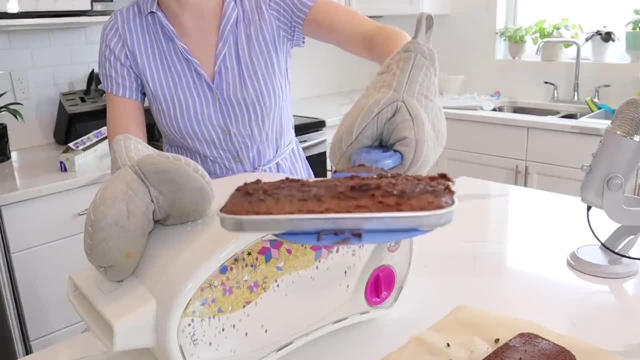 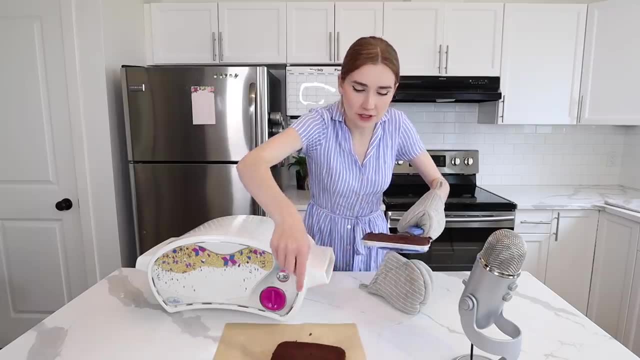 why does everything go so high up? Look at it, It's scraped. I mean it feels done. I think not really, Not really. I have this one down here and this one, we'll be able to make something work. Okay, This has been some movie magic. I actually just got back. 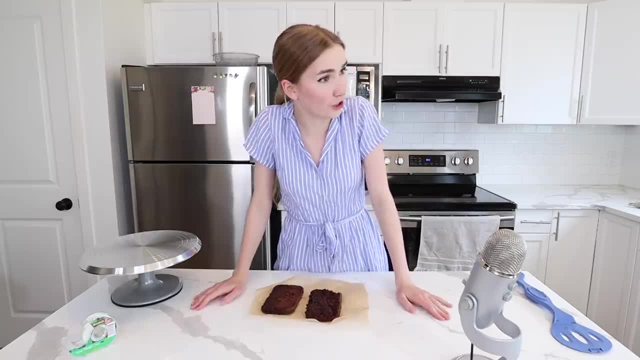 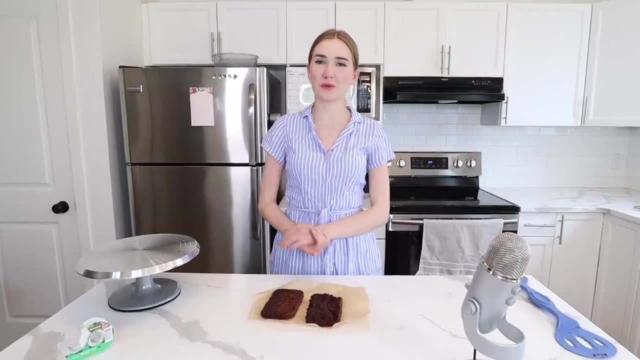 From my naturopath appointment and I have to go off sugar for an entire month and blood work, which I just did five minutes ago. So this is going to be my last living it up. but okay, These were in the fridge the whole time, So they're cold now. Very nice, Very nice, Okay. 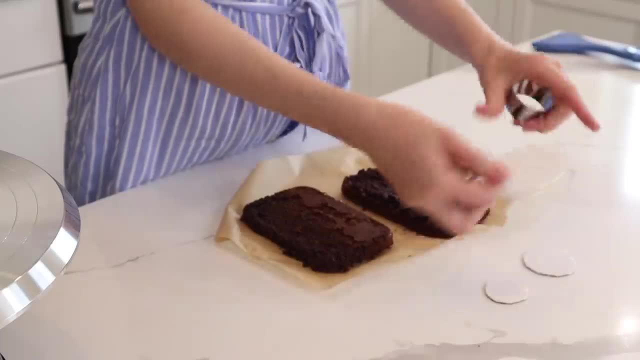 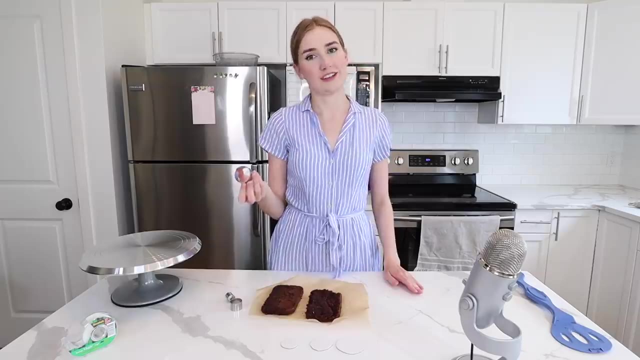 So I just made these little cake plates, because usually you would put your cake on a little board. So I made those. and this is when we're going to do this little cookie cutter. So let's do it. I almost feel like that might even be thick enough If I cut those all in half. Oh my gosh. 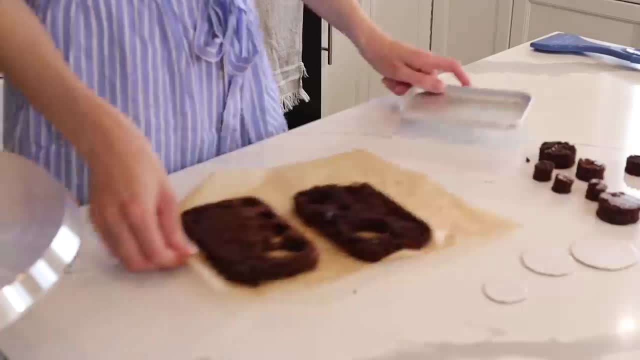 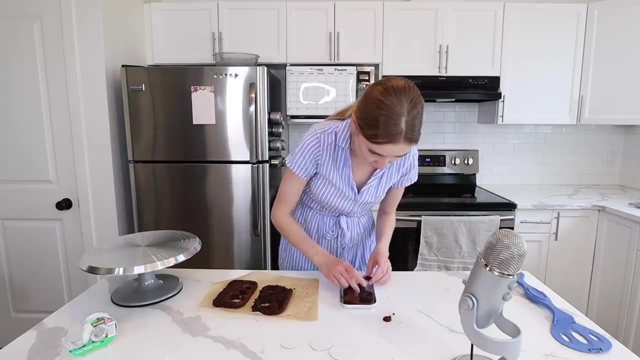 It's so small It's like hard to use my fingers. Okay, I'm going to put my test subjects in here. They're the ones I'll be working with. I just ripped this one in half. Now, I know this knife may seem overkill, but I need to cut these in half. 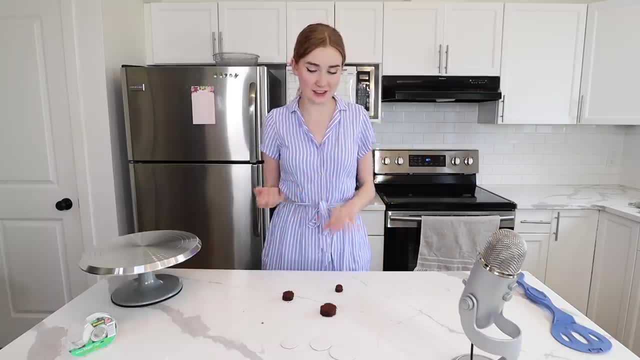 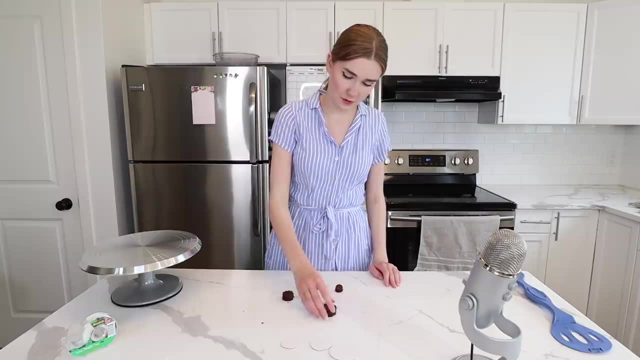 This feels so funny. I I actually was initially when I was planning this video. I was going to make a dog cake, like a dog safe cake, Um, but I didn't. So if you guys want to see that, we could definitely make one. but here are our pieces. Now we must ice them. 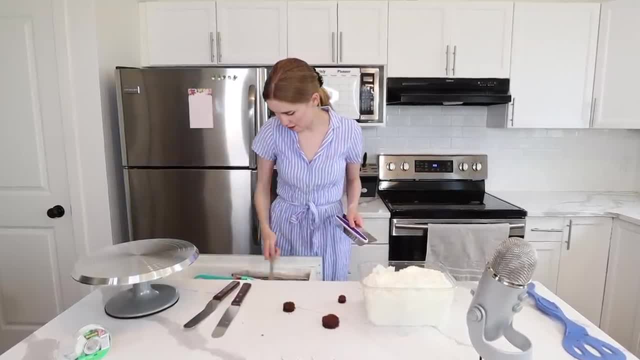 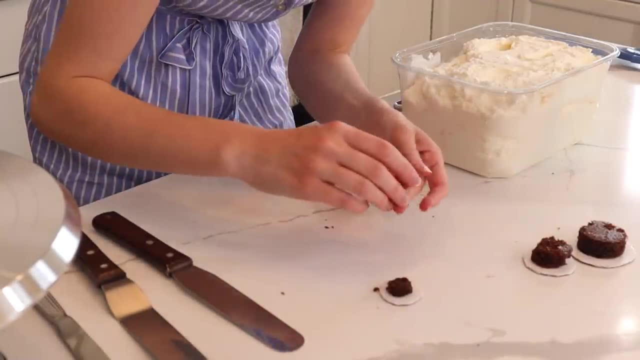 I only have these giant spatulas. Oh my gosh, This is not going to end very well. Oh my gosh, This is so difficult. It's so small. So I have this big tub of icing, pretty excited about it. So good, Got a new metal. 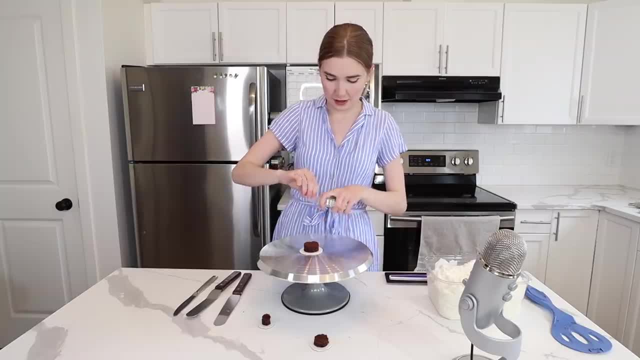 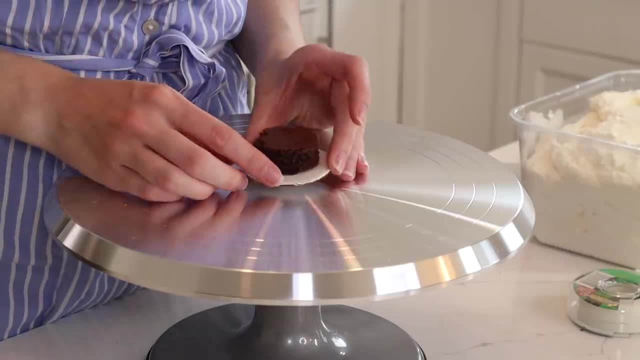 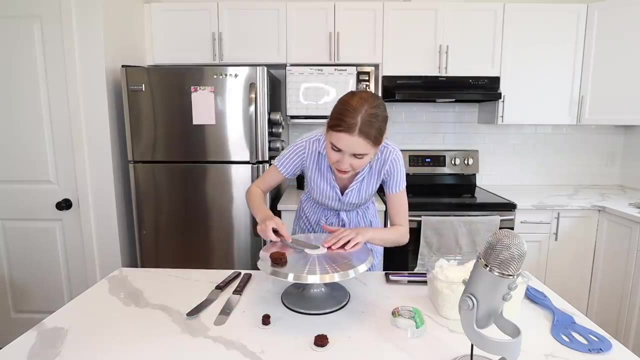 Spinning tray. Ooh, Firstly, by taping this little plate to the spinning turntable thing. You guys told me this would make my life a lot easier. So I'm listening to you guys. And then you also said: if I put down a little bit of icing, it'll kind of act as glue. 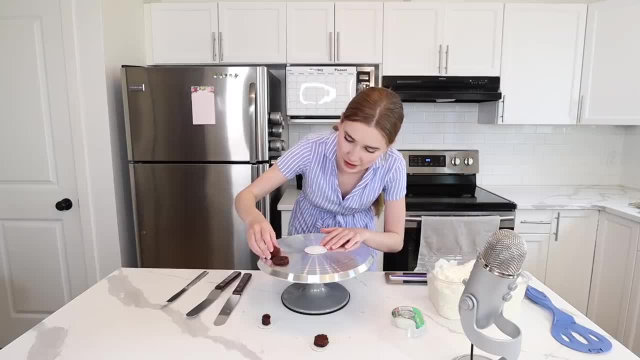 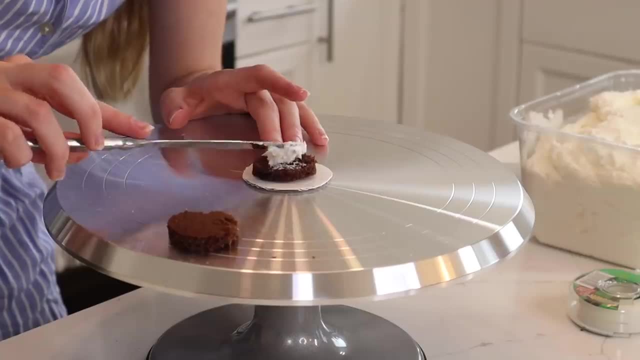 So again, I'm listening to you guys. You guys are the experts, So I'm just going to put that down. It is so small I feel ridiculous. Oh my gosh, The icing's like a little bit too big, Too cold. I'm just going to warm up a bit of icing just because I don't want to rip up any of 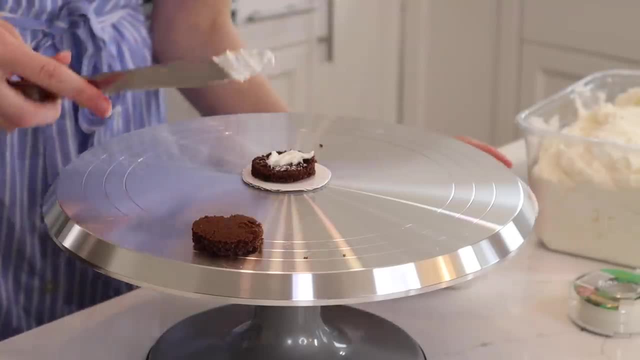 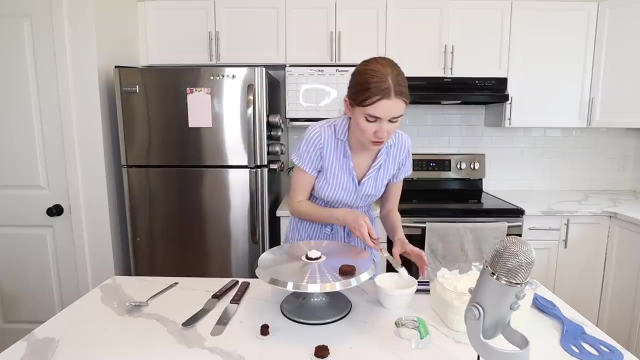 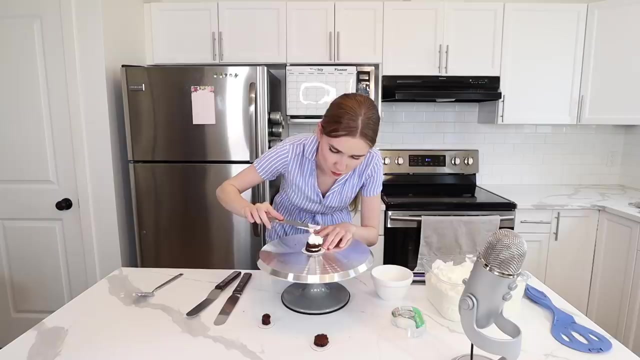 the cake. Oh yeah, That's warm. now Let's go ahead and just do the icing in the center. Now, this is my first time doing layers. I don't know why I chose today for the first time, but I did. It's so cute. Now I'm going to do a little like icing coating. Oh my gosh, I just have to be. 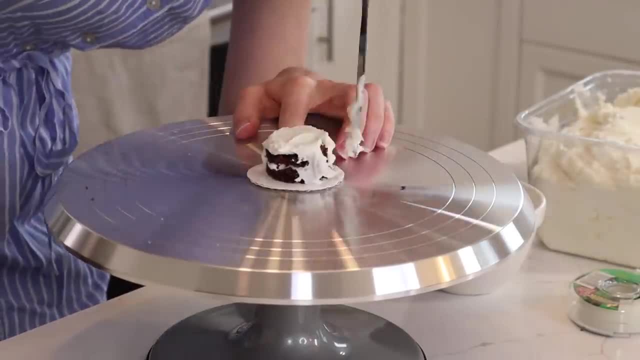 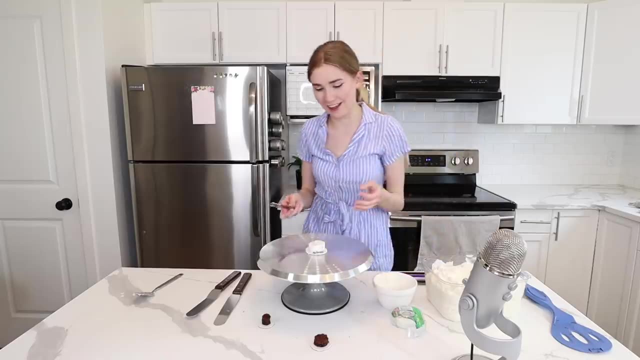 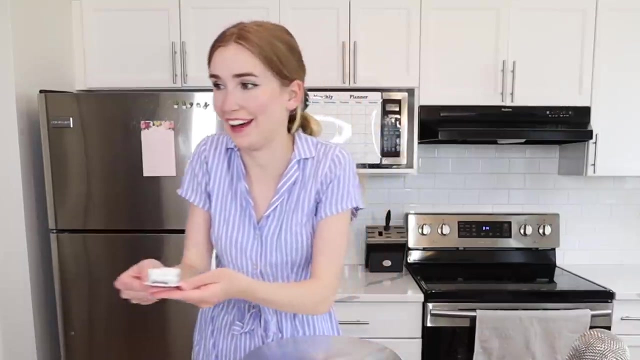 patient. Oh my gosh, I actually feel like that looks pretty good. It moved around a fair bit on the plate, but like, not bad. Here is what my crumb coating looks like. This is the biggest piece, So I'm a. 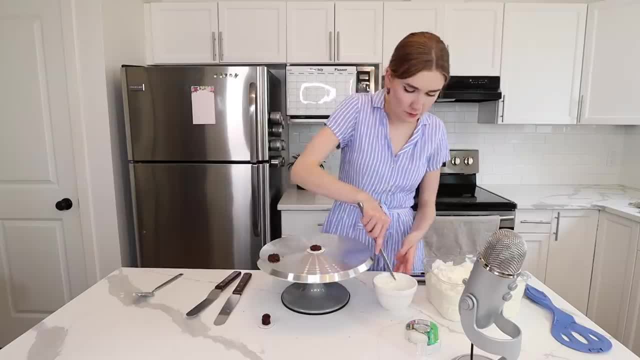 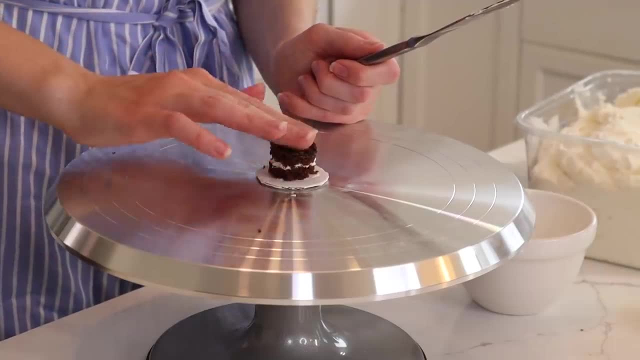 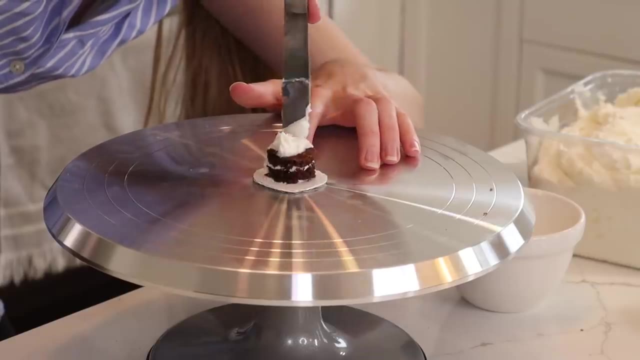 little bit concerned. Right on top of the pickles, I'm obsessed with caking. I love it. So fun, So tasty, Oh my gosh, It's so cute. All right, Crumb coating- Oh my gosh. This is so small, It's moving around so much. Oh my gosh. 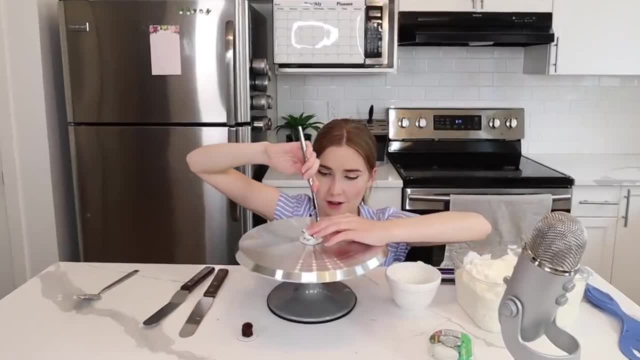 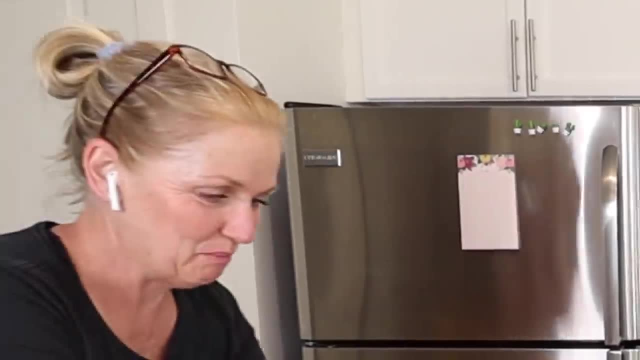 I can confirm. This is definitely harder on. the smaller one. Are those dental tools? Don't be shy, Didn't want to bust in, but we have science tools for these, Thank you. Thank you, That'll be good Oh. 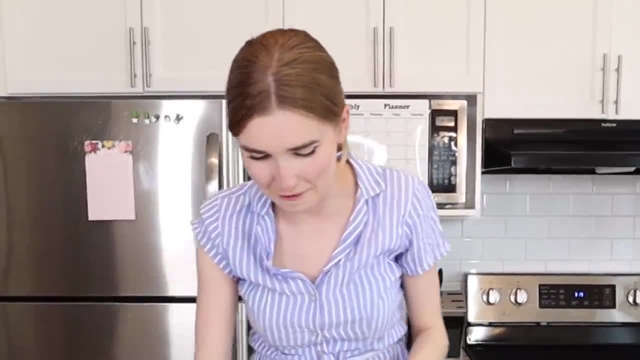 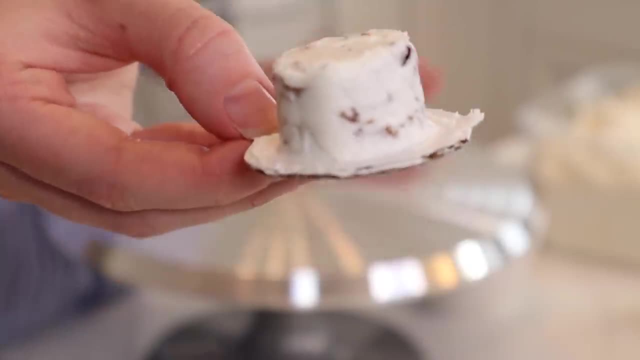 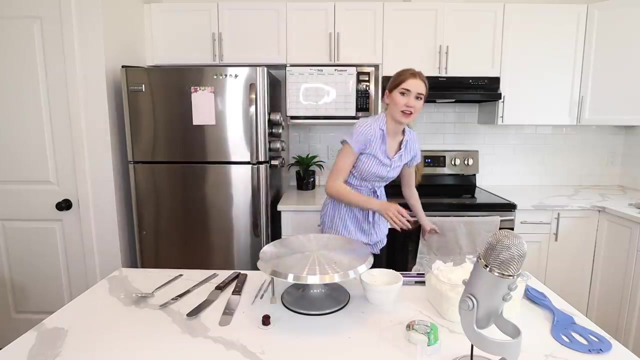 It's okay. Okay, Here's the medium layer. Now we have to do the smallest layer. Oh my gosh, They look so ridiculously cute in there. By the way, it's okay that I'm licking my hands a bunch, because I will be the one eating these, So don't be scared. Time to do the smallest one. 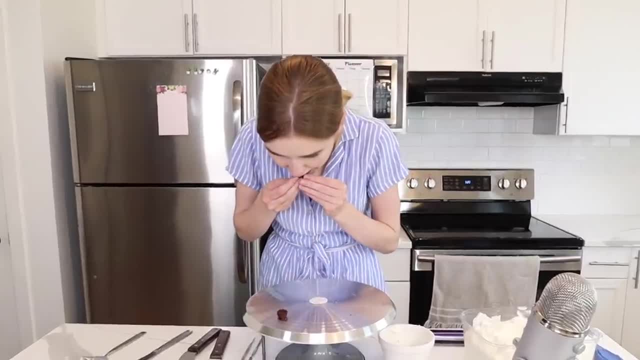 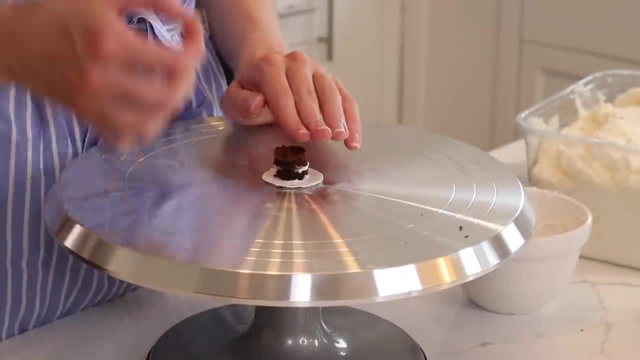 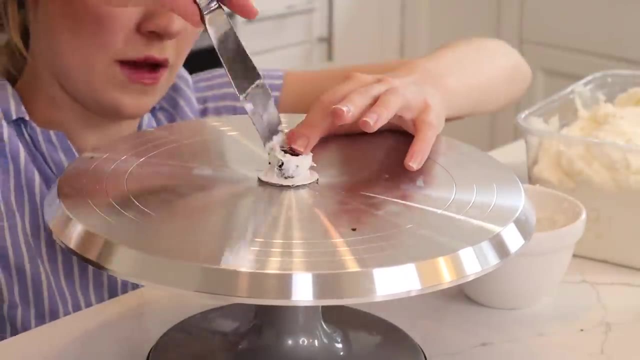 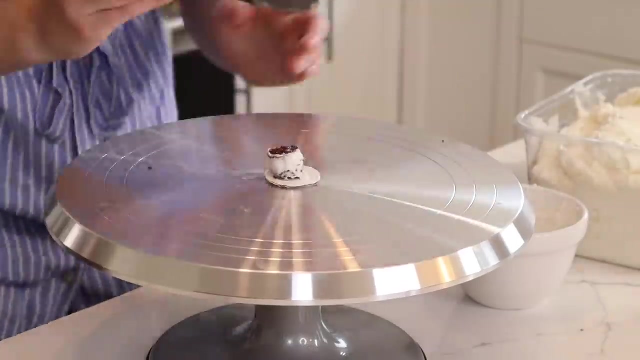 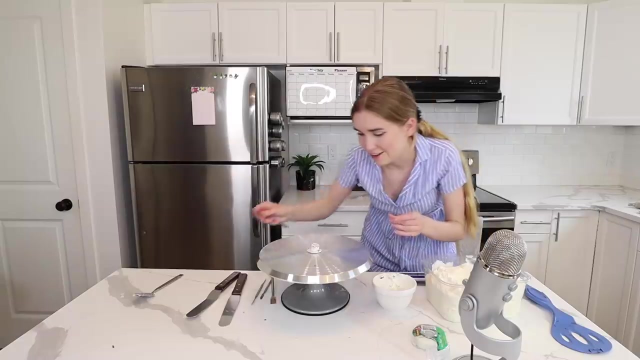 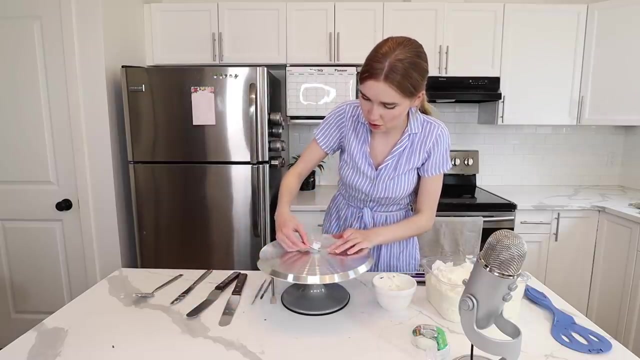 It feels a little too thick on the bottom. Hold on, No, that's better. Oh my gosh. Okay, That's as good as that one's going to get. I think It's a good enough crumb coating. This one's really hard. It's like so small, All right, Here's that top layer in comparison to my thumb. 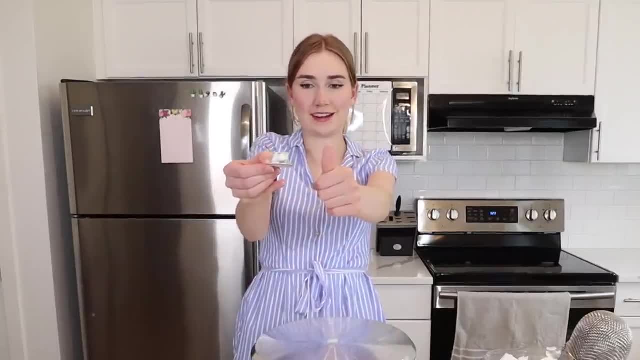 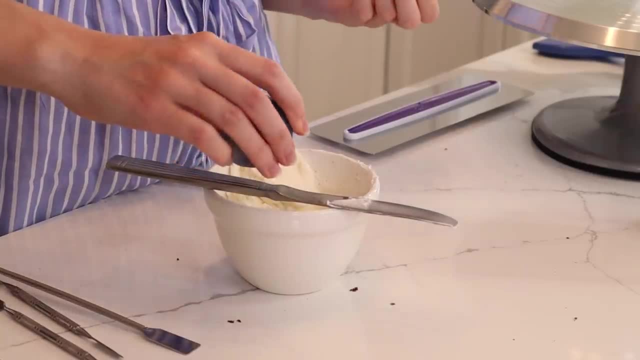 Here's how big it is. So, yeah, I don't really know what to do, but I feel like a very safe bet is a light pink. So light pink, almost white. So I'm just going to do one drop of this red food. 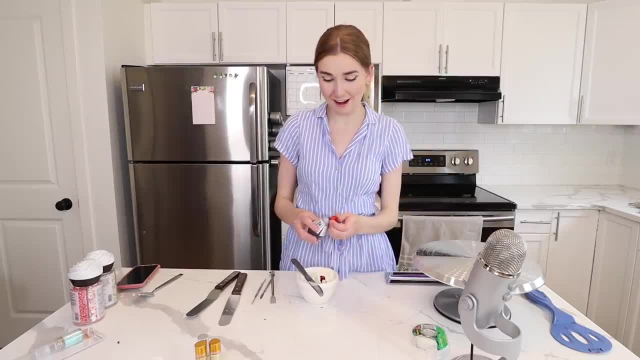 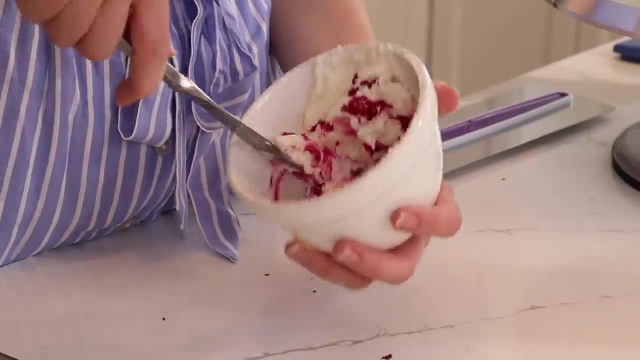 coloring. Oh my gosh, We're doing a red cake today, apparently. Okay, Let me just see what I just did. Maybe this will be the answer. OMG, you guys, Look what I just did. That came out a lot. 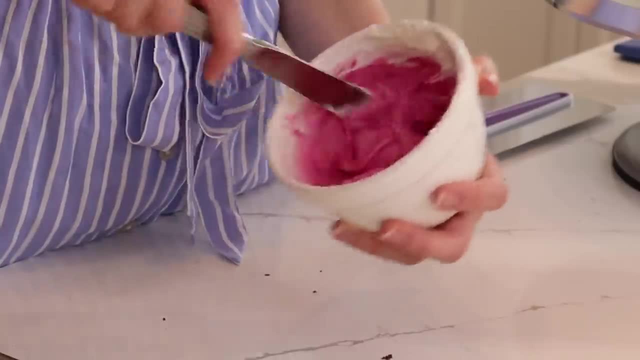 quicker than I was expecting. I'm going to do a little bit of a red food coloring. I'm going to do a thing to protect it. That's not what I want. No, Hold on just a minute, I'm just going to grab. 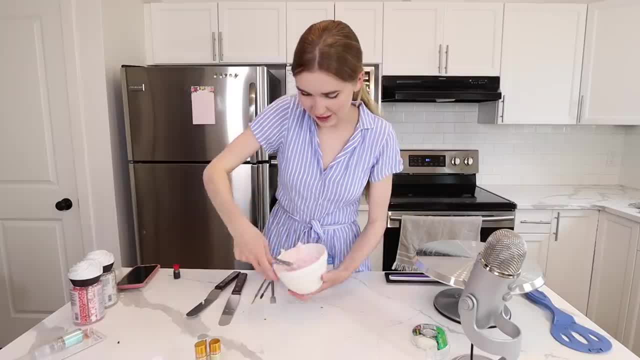 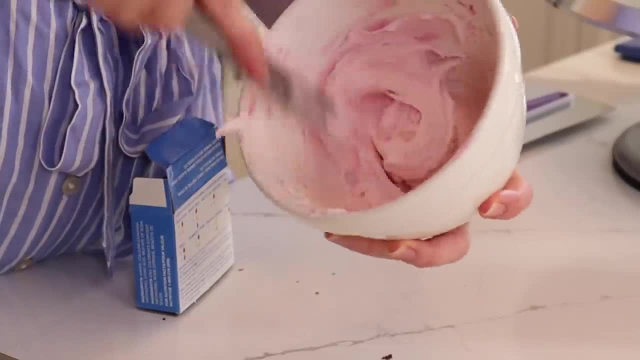 some new icing. Oh, that was stressful. I feel tempted to put sparkly pink in here. Is this a bad idea? Probably. Oh well, I'm doing it. Ooh, I'm just basically going to coat these again. Oh my. 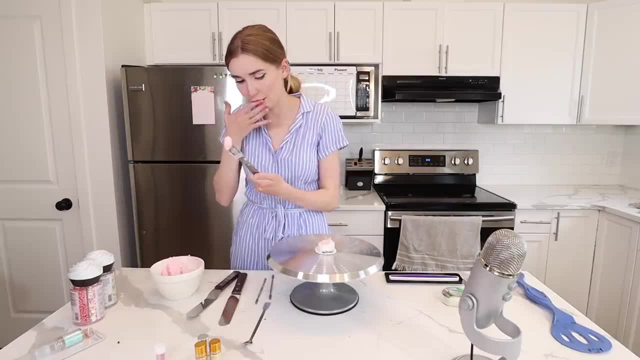 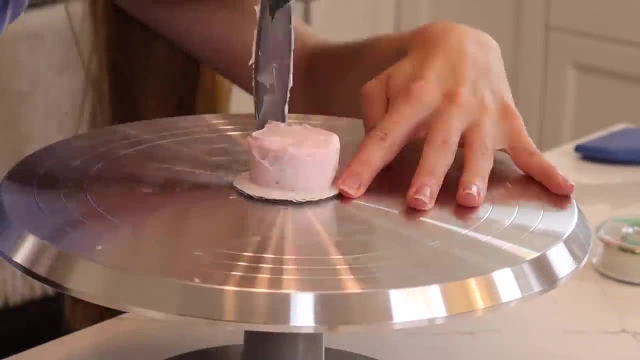 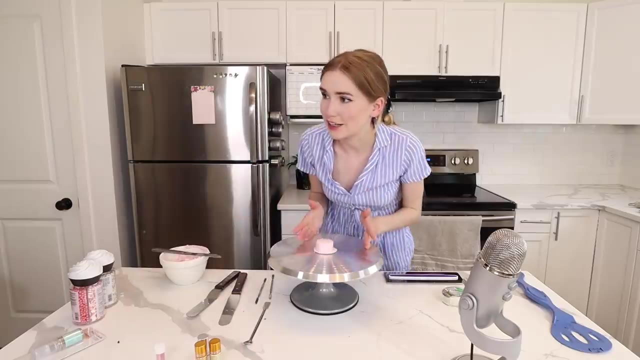 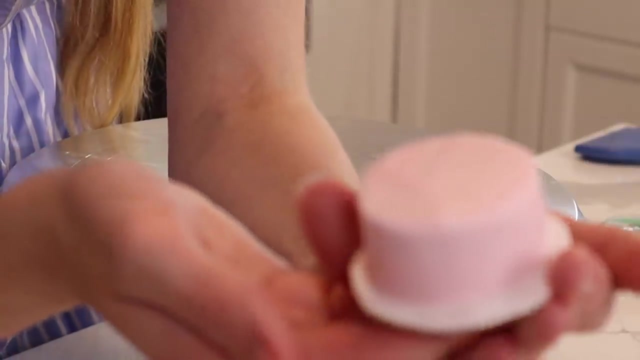 gosh, this one's going to be way easier because it's actually stuck down. all right, that's as good as i can get this. it's so flat in my opinion. oh my gosh, whoa, who's impressed. that's not bad. that was also the easiest one. 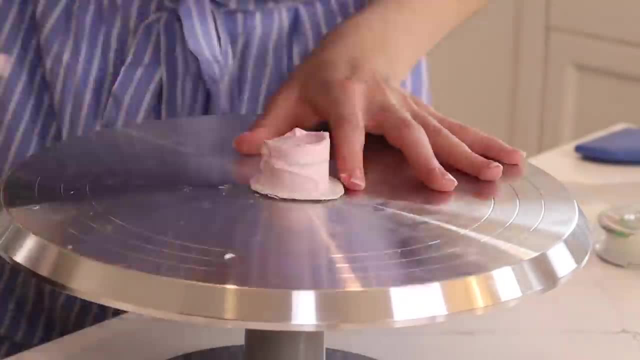 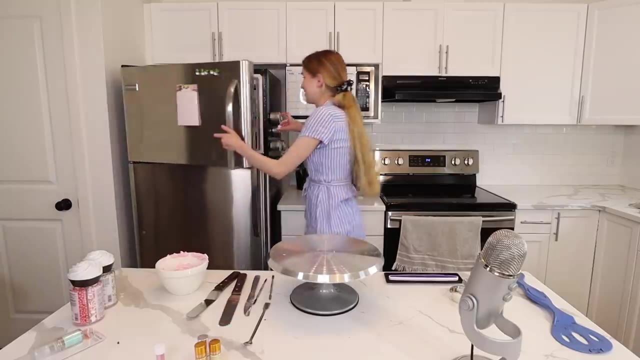 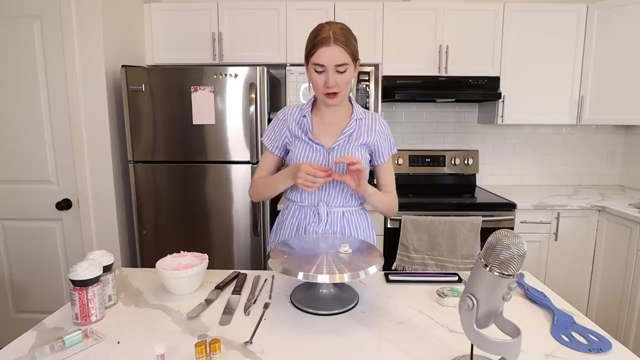 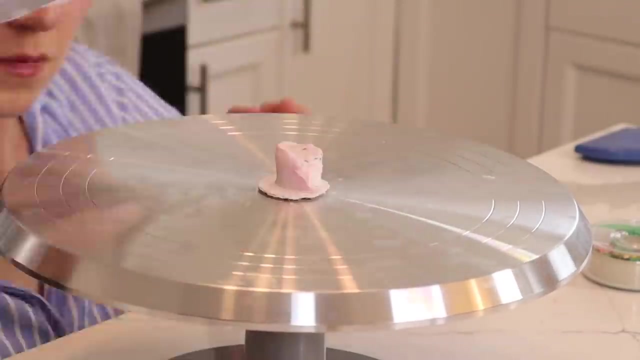 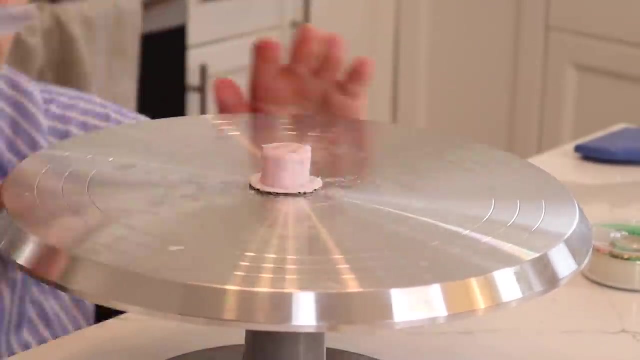 last one. they look so cute in there. oh my gosh, i can't handle this. i can't handle it. it's also getting dark out now. it's very late. last one, let's do this. no, turning back now, i'm very afraid for this next part. i have to stack the cakes. i just don't want to ruin them now. 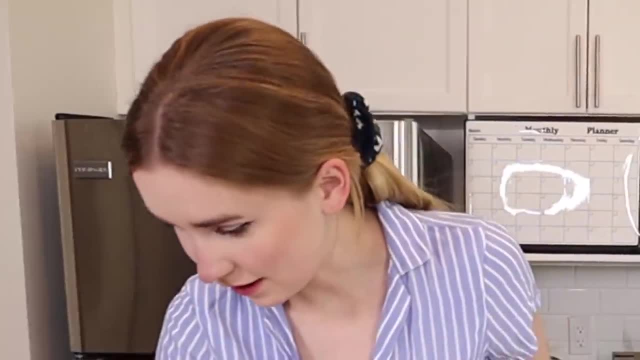 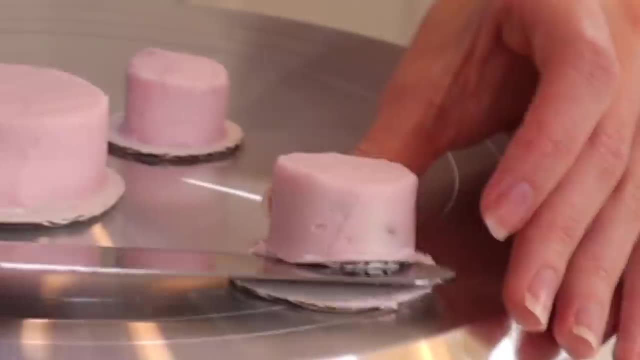 oh, i cannot get over this, but i'm scared because i don't know how to do this. i don't know how to cut them off, maybe like this. this is what i would do with a normal cake. oh my gosh, oh my gosh, oh my. 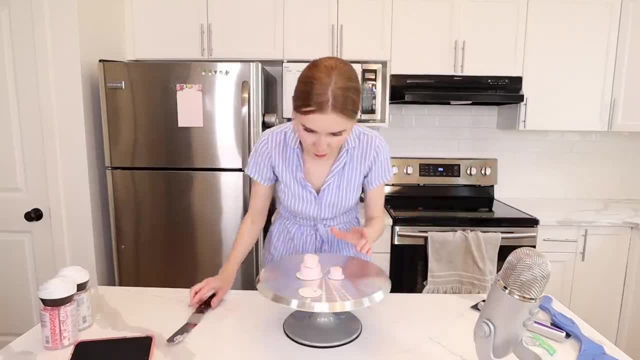 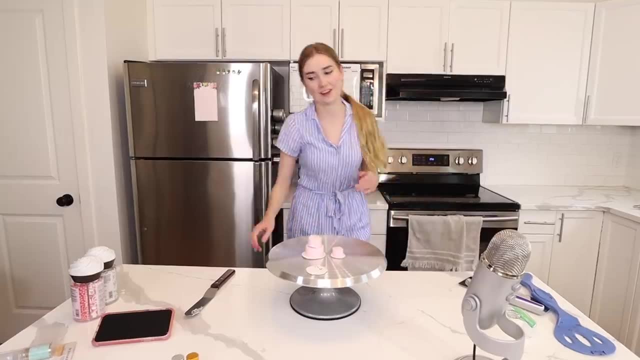 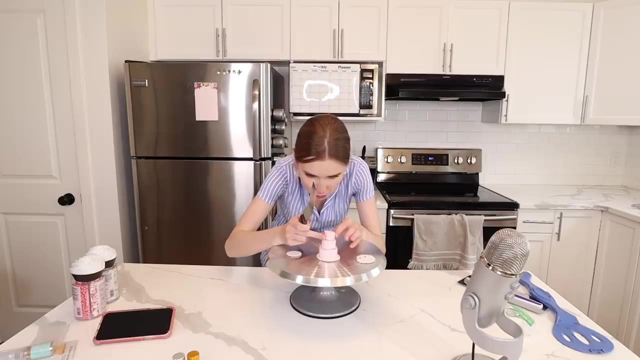 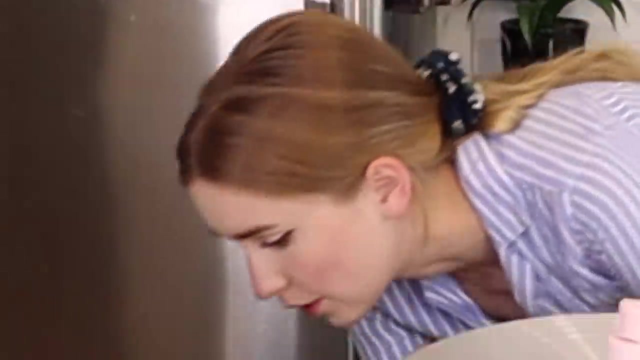 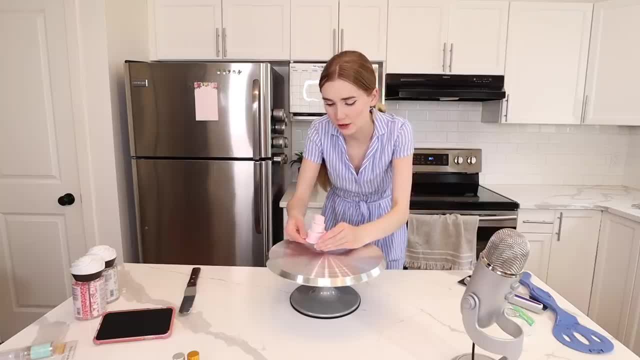 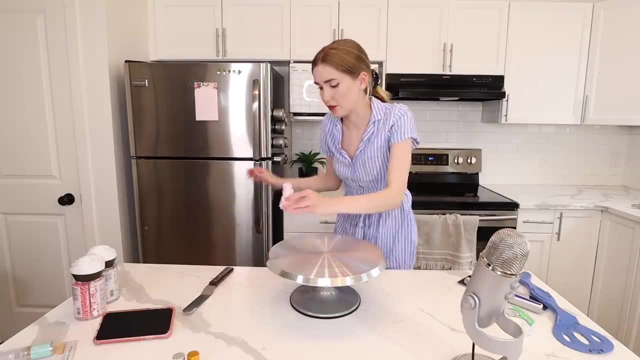 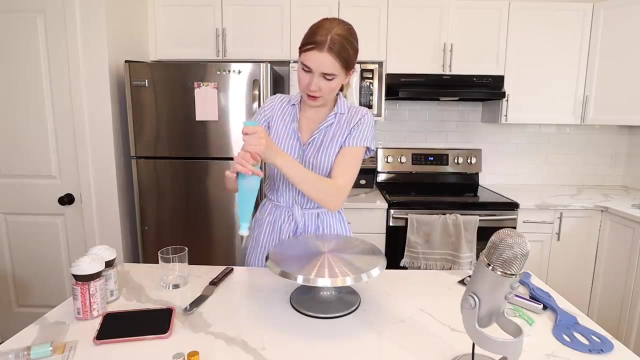 the layers. i feel like it'll be okay. let's just push it down a little. stay on there. what am i doing? i'm so stupid. oh my gosh, go in the fridge, go in the fridge, stay in there, don't do anything silly. okay. so we got that leveled. i put like a little tip on here. i'll. 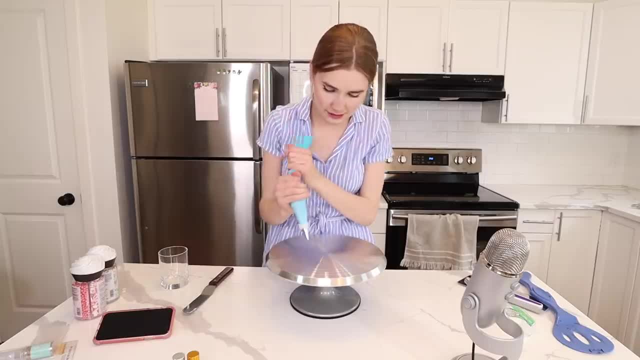 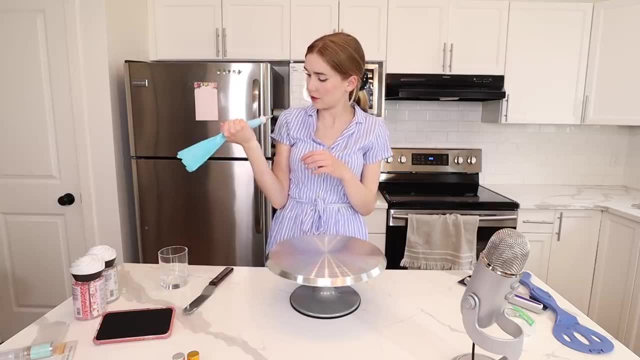 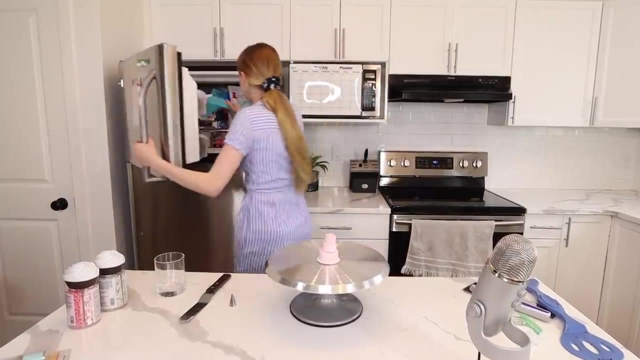 show you it. there's so little icing in here, but let me just test and see. i'll test it on my hand so i can eat it. whoa, that was not what i was expecting. to be honest, i don't like this tip. i need to swap the tip. okay, for real, this time it's way too warm. what is up? sorry, excuse me. 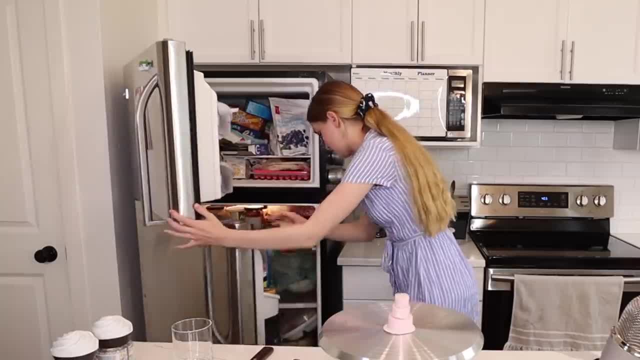 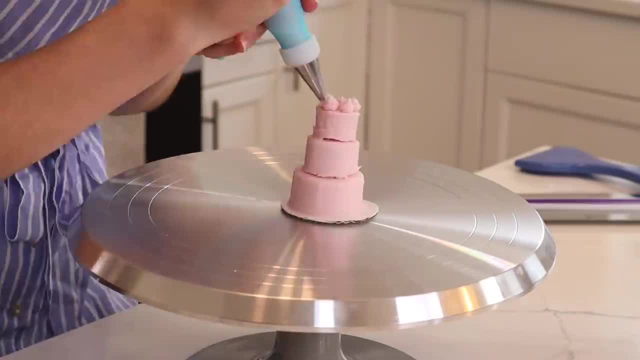 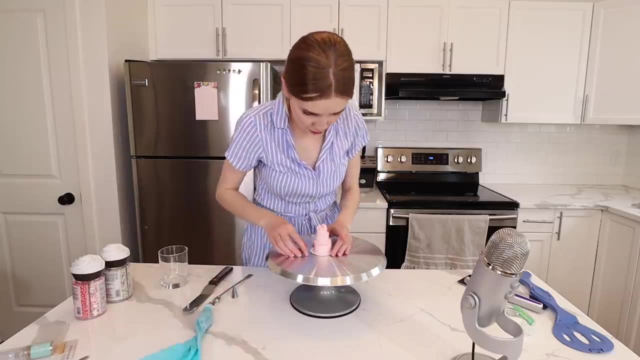 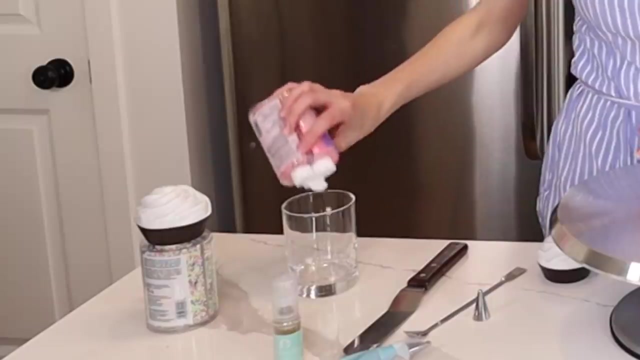 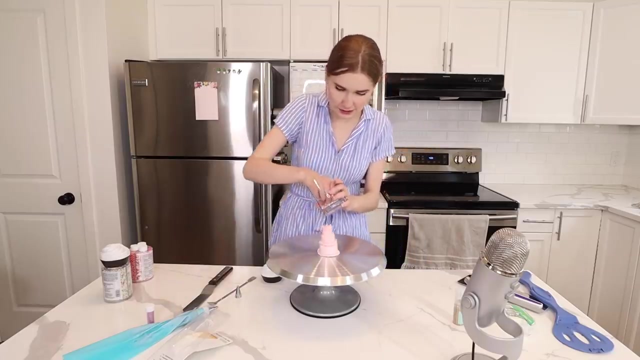 i just need to let that cool fell down. get in there. okay, let's do this. i want to start with the top. it's got to go in the fridge. another frozen banana flying out. let's just finish it up before we ruin something. a little bit of glitter for safety now specifically placed sprinkles.